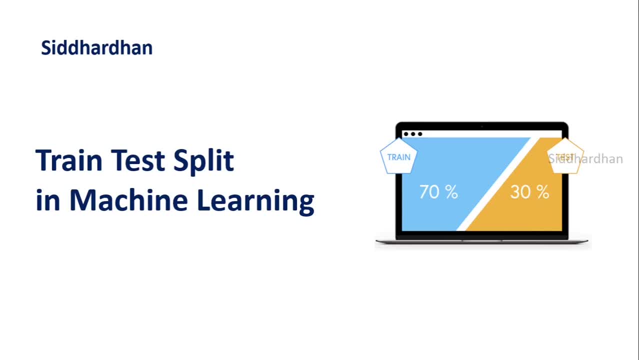 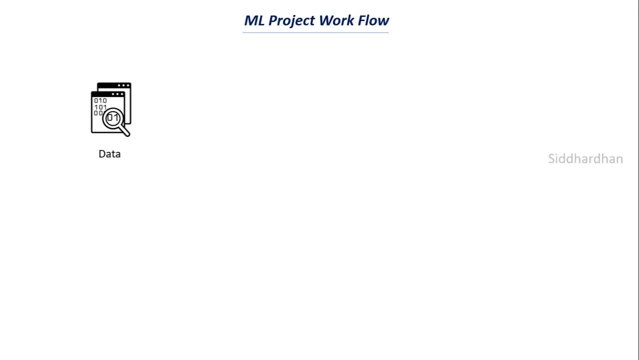 the general workflow which we will follow in a machine learning project. So this is how a machine learning workflow will look like. So the first step in any machine learning project is to get the data we want. So this data is chosen based on our problem statement. 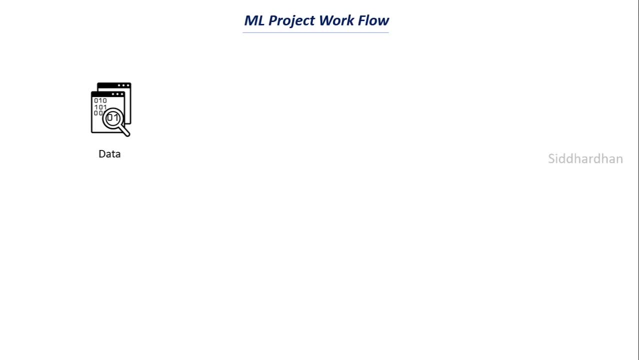 So let's say that we want to predict whether a person is diabetic or not. So in that case we want medical data for several persons, of diabetic and non-diabetic persons. So we use this data to train our machine learning model and do some predictions. So the first step is to collect the appropriate 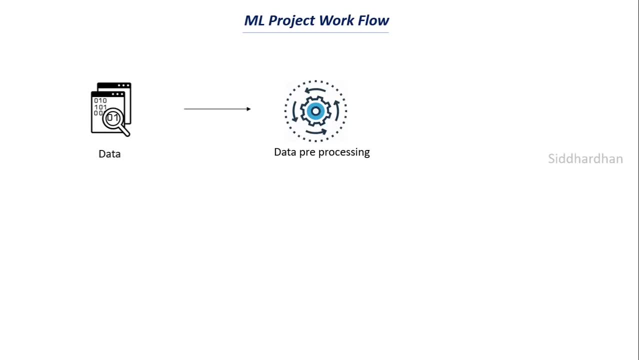 data. So once we have the data, we cannot feed it directly to our machine learning algorithm, So we need to process the data. So this is where data pre-processing steps come. So in data pre-processing we need to use some missing values to control the values of the missing data. For example, if the data has some missing values. 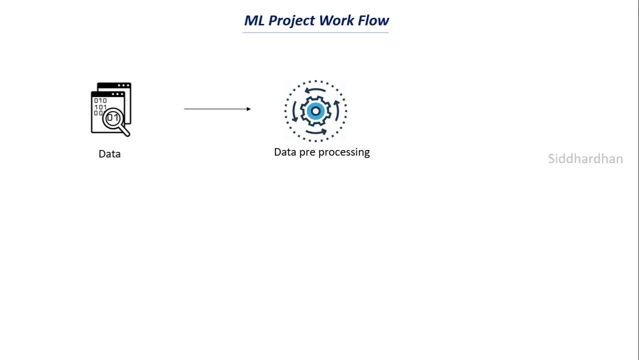 So we need to handle those missing values through some methods. So these are the steps that comes in data pre-processing. Okay, so once we do the pre-processing, we need to analyze the data. So it helps us to give some meaningful insights of that out of the data. So, for example, a data set may 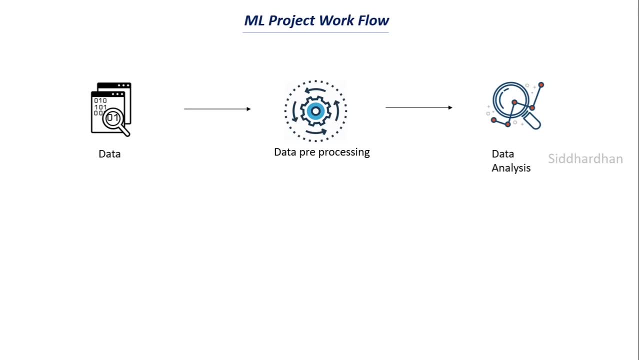 contain 10 columns or even 20 columns, so we call this columns as features. So we need to find which feature is important for the prediction and stuffs like that. So this is where we use data analysis. so in this we, you know, make some plots and analysis to see which features are. 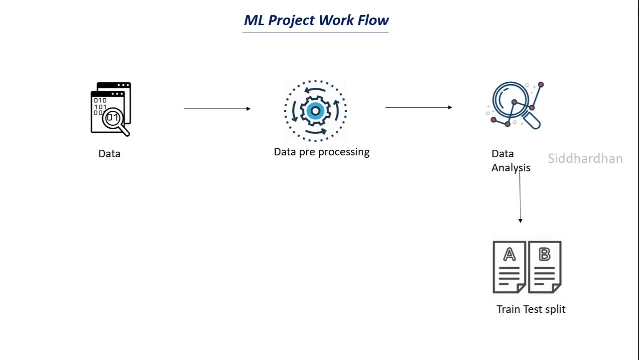 important. okay, so once we analyze the data, the next step is to split the original data into training data and testing data. so this step is known as train test split function. so this is what we are going to see in this video. so, once we split our original data into training data and 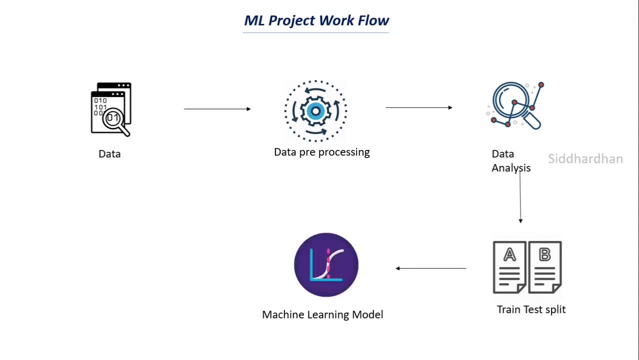 test data. we will feed this training data to our machine learning model. okay, so there are several machine learning models, so what we will do is this: training data will be used to train our model, so our model will find the pattern and learn from this training data. okay, so, once it has learned, 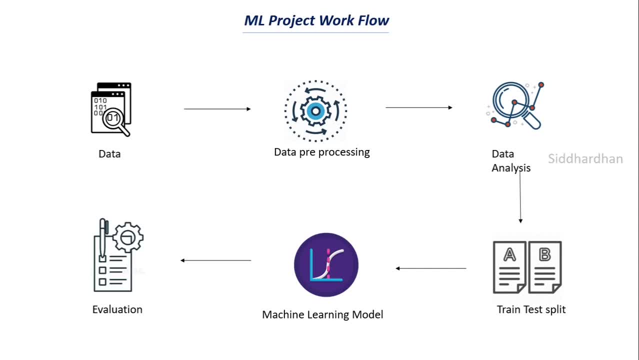 from the training data, our model will be evaluated, and this evaluation will be based on the test data. okay, so evaluation is about finding how the model is performing and what is the accuracy score of the model and such kind of things. so the takeaway is that we use the training data for training the 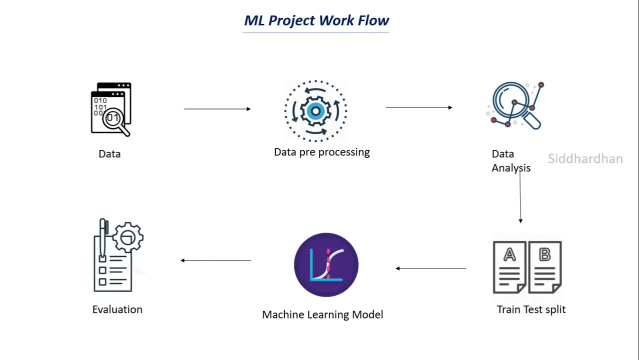 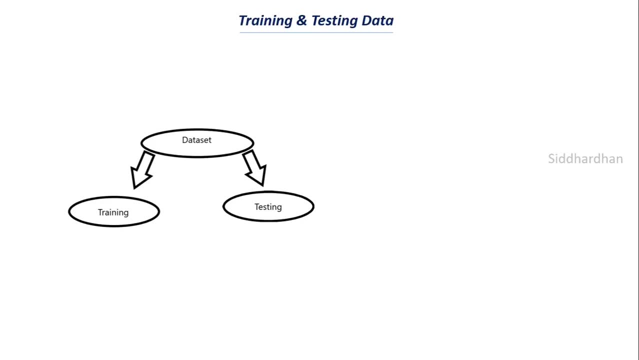 model and we use this evaluation by the training test data. okay, so now let's see what is this train test split? okay, so when we have this original data set, so we take 80 percent or 90 percentage of the data as training data and we take 10. 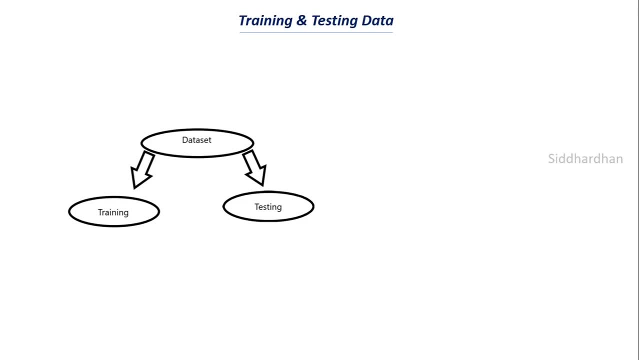 percentage or 20 percentage as testing data. okay, so which is used for evaluation? but what is the need for this evaluation? so let's try to understand this with an analogy. so let's say that a person is studying for a max exam- okay. so let's say that he is preparing- uh, you know- for 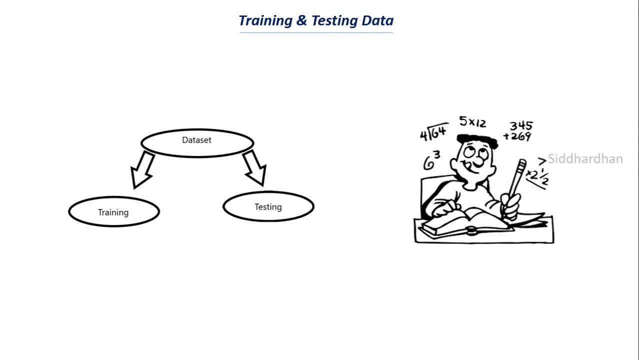 the exam by practicing the questions and given in a textbook, so that questions will become the training data. so in exams the examiner will ask the questions that may be out of that book. okay, so because if, uh, the questions are asked out of the book, then only we can, you know, evaluate that. 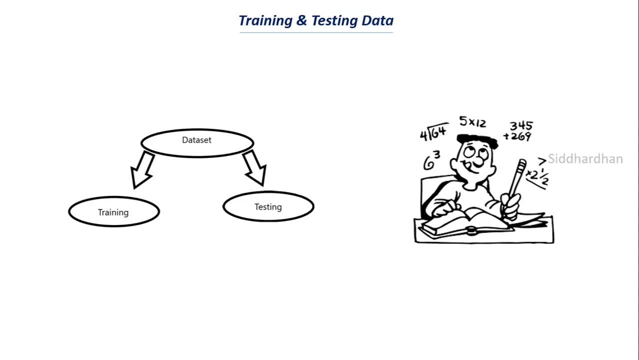 the person has studied well, okay. so asking the same questions given in the textbook may not be a correct metric to you know, analyze his performance. so this is the same example here, so based on the training data, because our model has already learned, has already seen the training data. 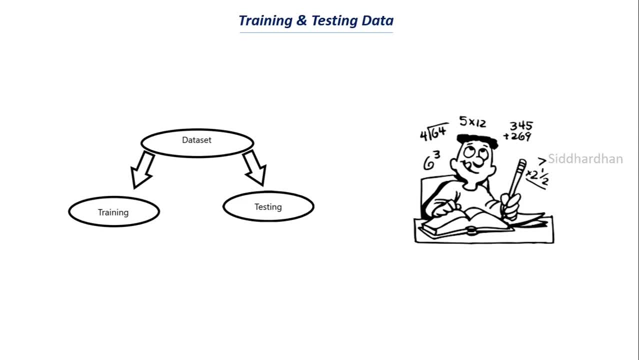 but it never saw the test data. so that's why we need this testing data: to evaluate our model on how it's performing and what is, uh, the accuracy score and other metrics of the model. okay, so, with that being said, let's get into some coding part and how to do this. training and test testing split. 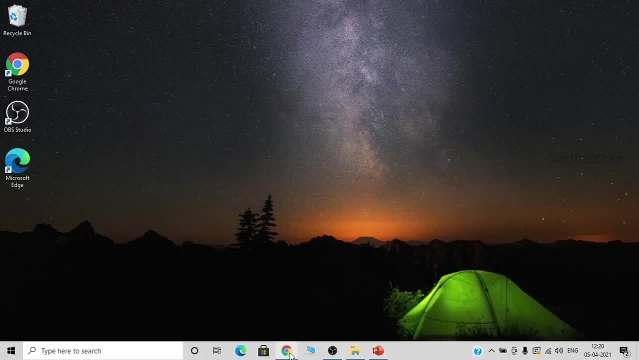 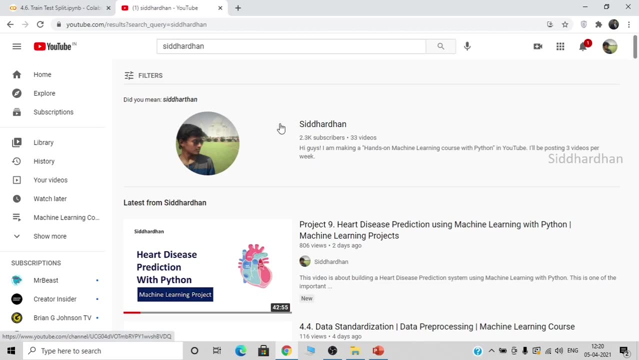 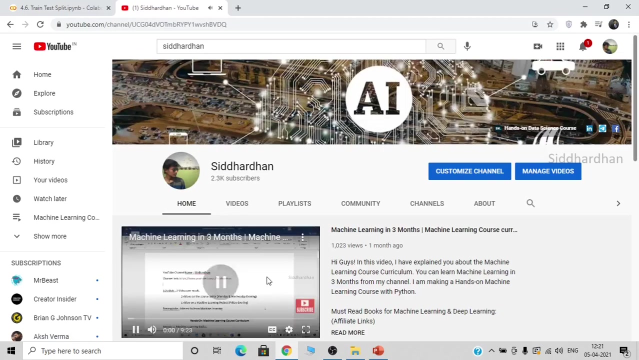 okay, so i will be doing this in google collaboratory. so before starting with the video, i'll just show you a quick intro to my channel. so this is my youtube channel in which i'm posting my machine learning videos. so once you go to my channel you can see this machine learning course curriculum. so in this i have explained about all. 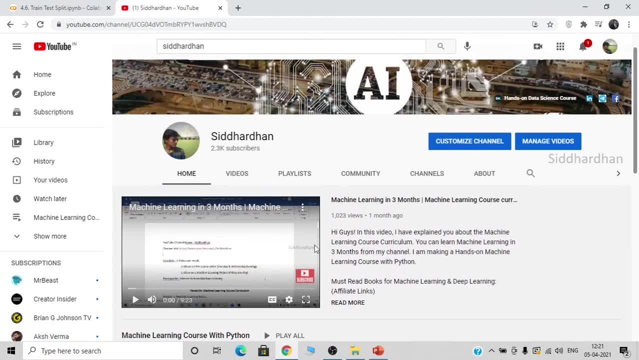 the modules and the videos that i will be covering in this channel. so in the description of the video you can see the curriculum file so you can download it and go through it. so i have also mentioned some important machine learning books that you can read. okay, so it is also given in. 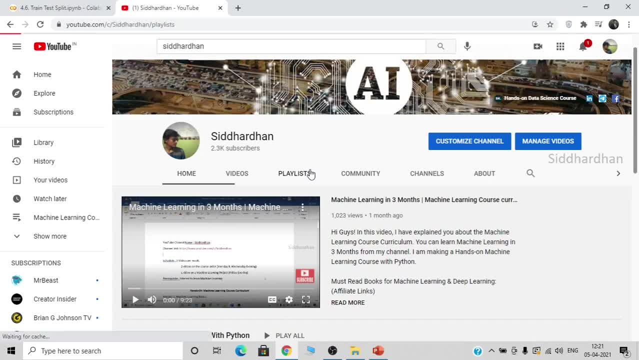 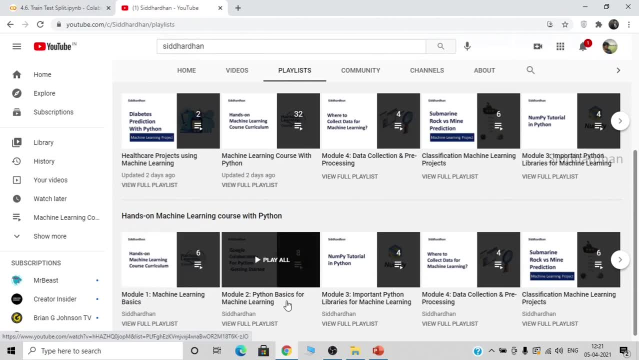 the description of all the videos so you can go to this playlist section to check out the modules. okay, so, as you can see here, the first module is on machine learning basics. the second module is on python- basics required for machine learning, then the important libraries such as num. 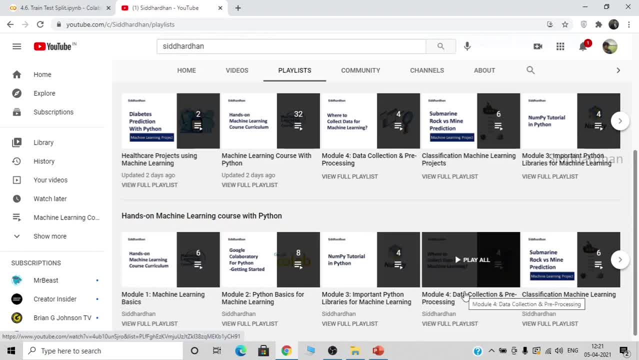 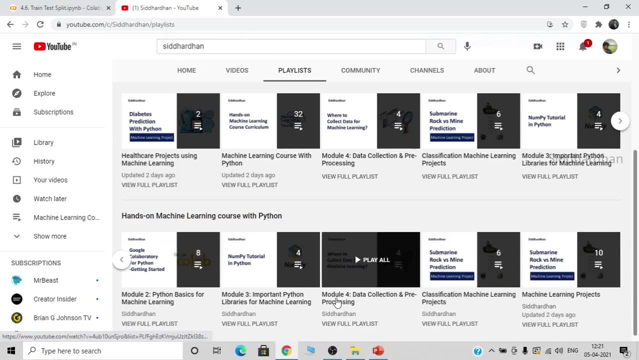 pipe, pandas, matplotlib and seaborn. okay, and the fourth module which we are discussing right now is data collection, pre-processing and also i have several machine learning project videos, so i will be posting three videos per week. two videos will be on monday evening and wednesday evening, which 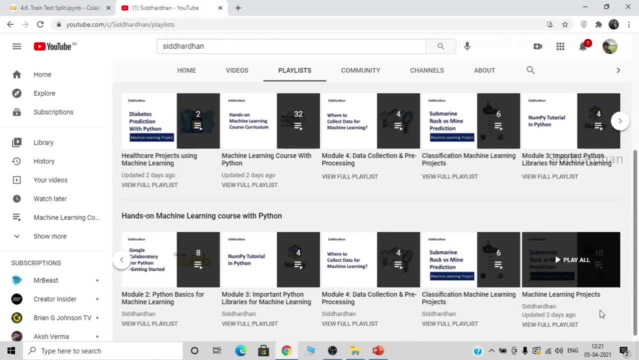 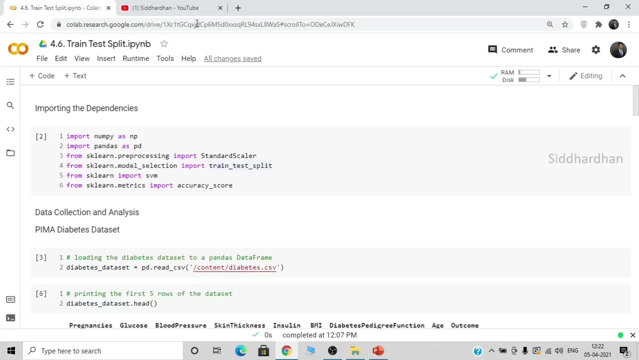 will follow this course order and every friday i will be posting one machine learning course video. okay, so you can also check this machine learning course with python. so i have, you know, incorporated all the videos in this particular playlist. so, in case you are new to this google collaboratory, you. 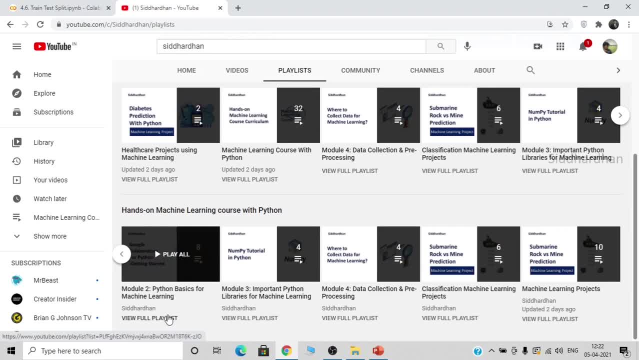 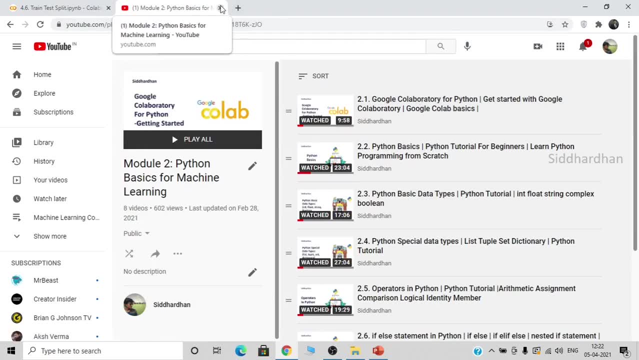 can go to the second module, which is python basics for machine learning. so, in that, the first video is about how you can access google collaboratory and how you can- you know- use different features present in it. okay, so now let's get into this section. so this is where we run our python. 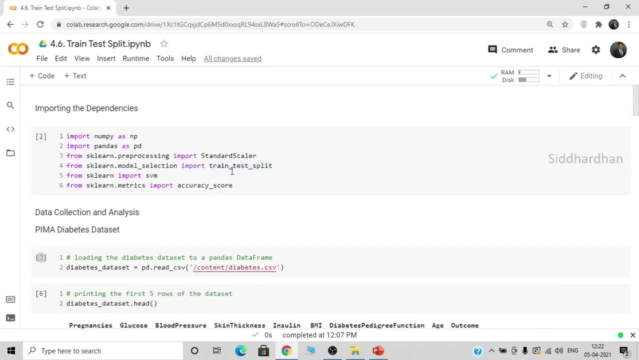 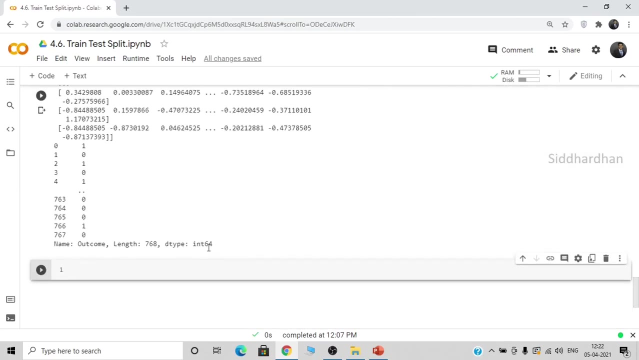 programs. so i have taken an example of this example project. so this is about diabetes prediction. so we have already did this machine learning project in our channel so you can go to the machine learning project playlist to see the full code there. so here we have the half code. so i will stop this video by, you know, splitting the. 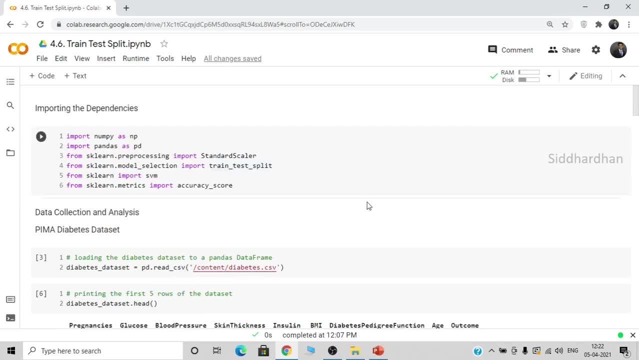 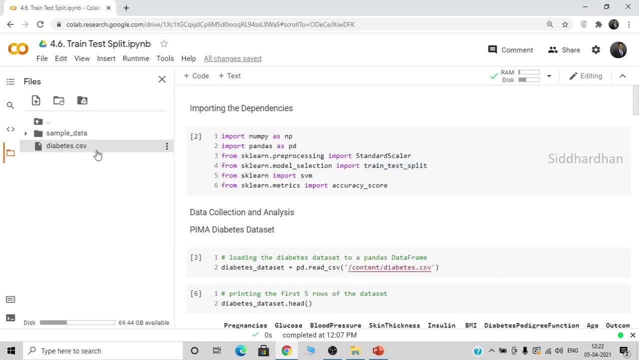 data into training data and testing data. okay, so before that i'll just give you a quick recap of what we have done here. so i have already uploaded the data set file here. so this is diabetescsv, which contains uh, the medicinal data. so i'll give the 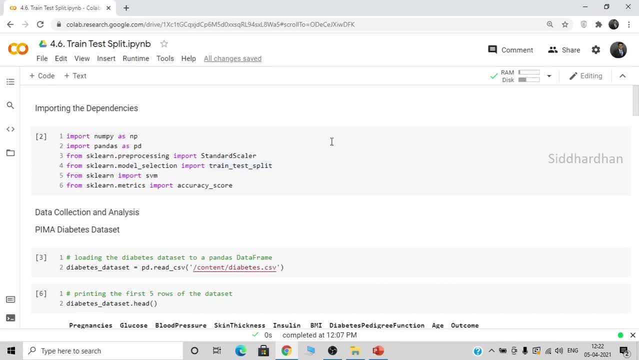 link of this data set file in the description of this video. okay, so first, what we are doing is: so we are importing the libraries, so we need some important libraries, such as numpy, pandas, escalon, so we use the standard scale function to standardize all the data and this is the train. 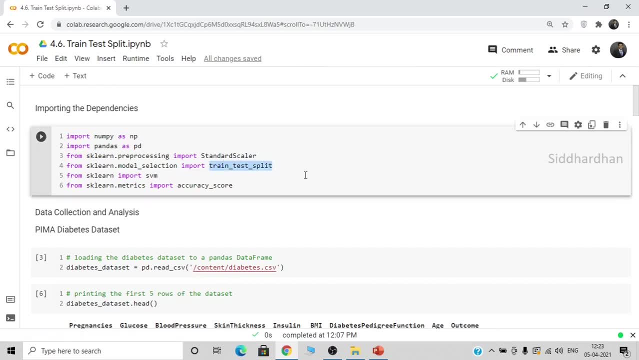 test split function, which we are going to see. okay, so this will automatically split our data into training data and test data. so in this case i will be using a support vector machine model for training and then we will predict our accuracy score. okay, so i won't be explaining, uh, the entire. 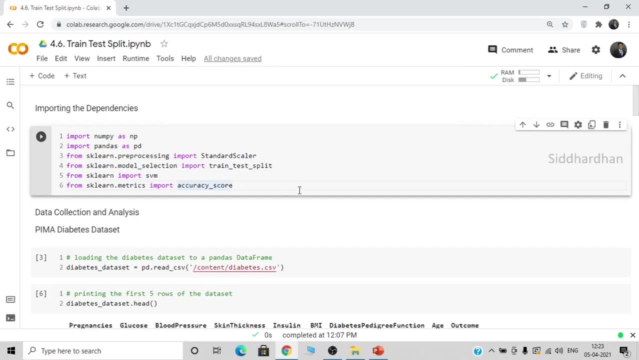 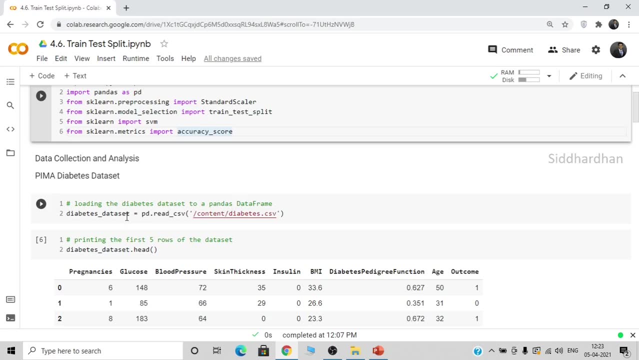 data set, because we have already did that in the diabetes prediction project video. okay, so i'll just explain this train test split function. so after that we have loaded this data set, uh, in a pandas data frame. okay, so, using this read csv function and we have seen what are the different columns. 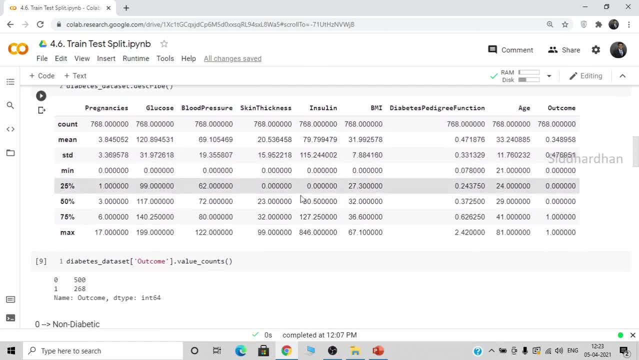 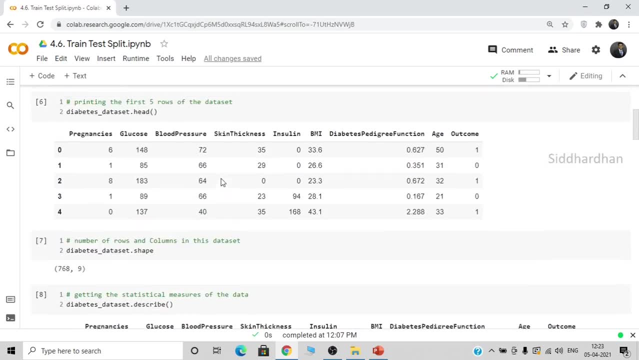 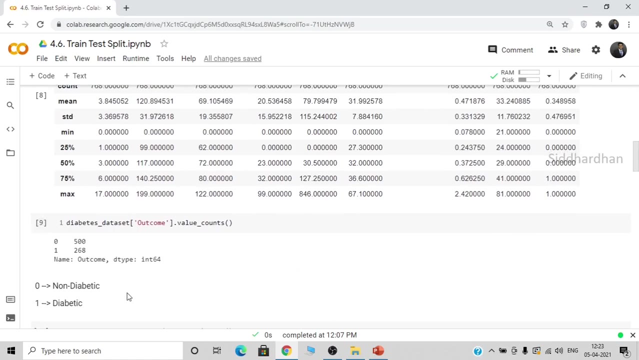 are present in it. okay, so these are some data analysis part on finding some statistical measures. and we found that there are two labels in our outcome column. okay, so you can see the outcome column here. it's either one or zero. zero represents non-diabetic patients and one represents diabetic patients. okay, 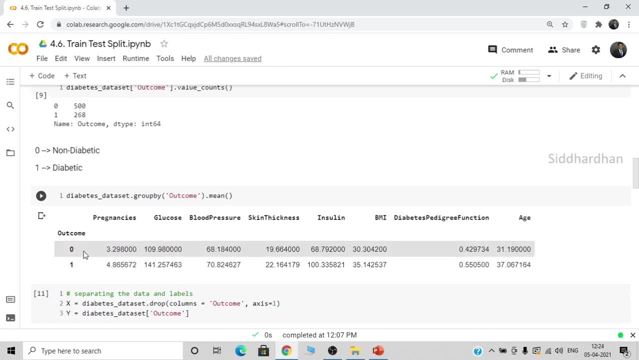 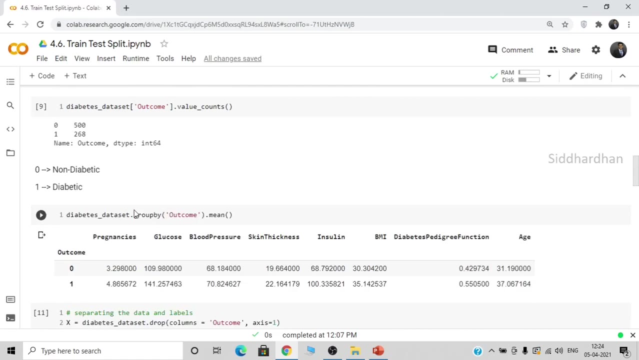 so you can see this is the mean for each cases. so for non-diabetic persons, this is the average value of each column and one is uh for diabetic people. okay. and then we are splitting our data into features and uh targets, okay. so the feature is all those columns except this outcome column. 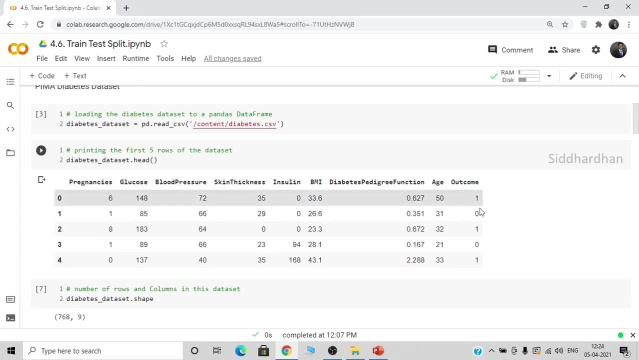 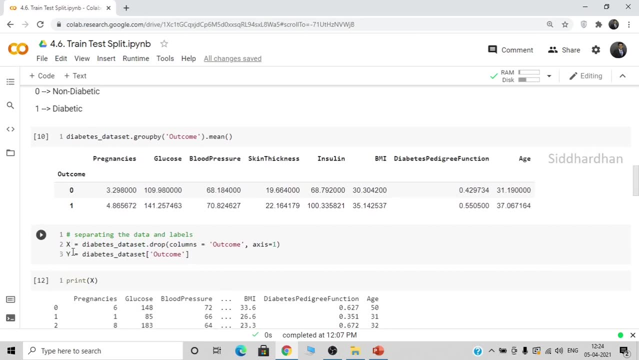 okay, so this outcome column is the target and we will take it separately. okay, and we have printed the outcome column in the case and all these other columns act as the features. so you can see, here we have stored all the features in x and all the features in y. okay so, and we have. 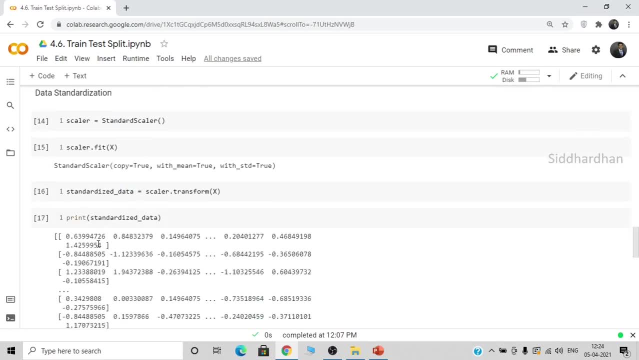 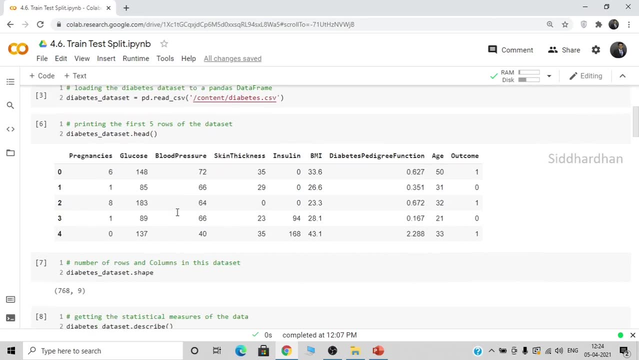 printed it and this x doesn't contain the outcome column and the y contains only this outcome column. okay then we have applied this standard scalar function. so this data standardization is used to make all the values in a common train. so you can see here. so some values are in the range of 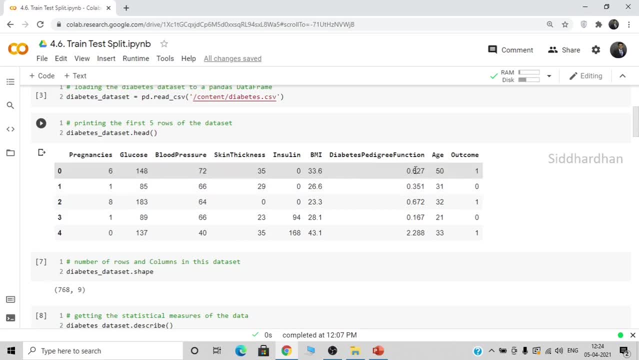 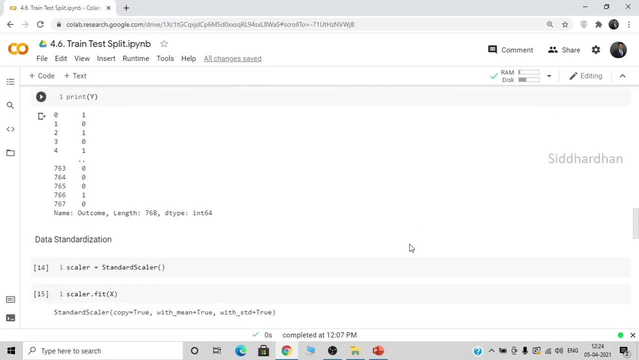 hundreds, and some are in the value of 20s and 30s, some are in the, you know, in the range of and such kind of things. so we use this data standardization to have all the values in the same range. okay, so we have standardized the data and the next step is where we will split our data. 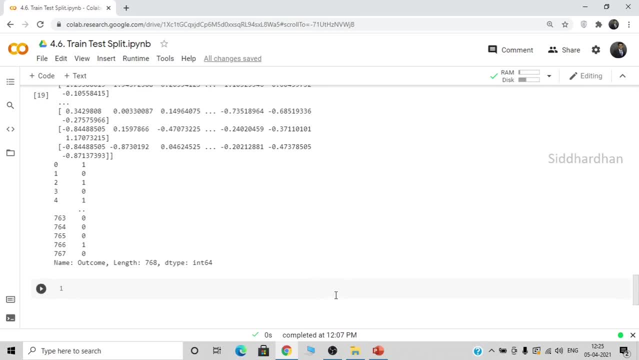 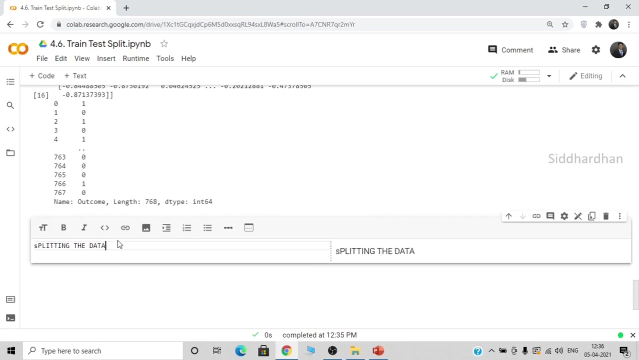 into training data and test data. okay, so if you want to know more about this particular project, please check out that diabetes video. so i'm not explaining much. okay, so now i'll just create a text here as splitting the data into training data and testing data. okay, so now we can use the train test split function that we have imported from. 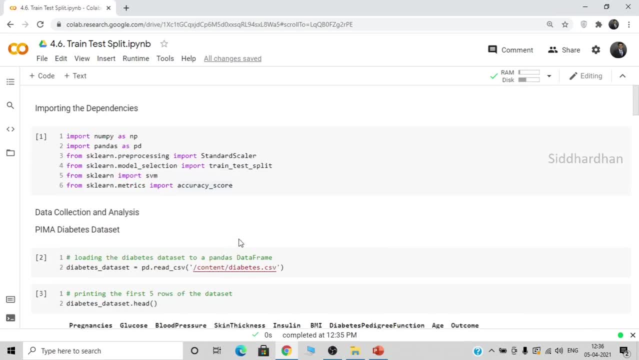 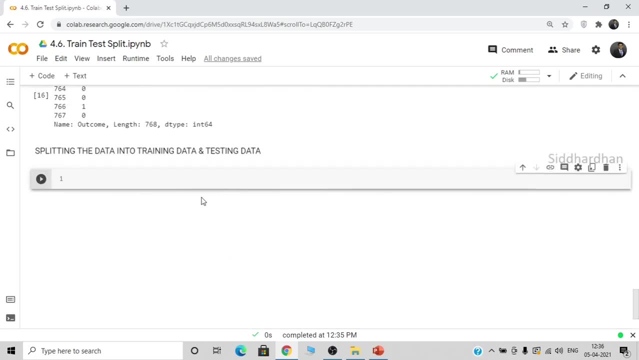 sklearnmodel selection. okay, so you can see this here. so we have imported this train test split function using sklearnmodel selection. so that's what we are going to use now. so before that, we need to create four arrays, so x train, x test, y train and y test. okay, so i'll just explain you what. 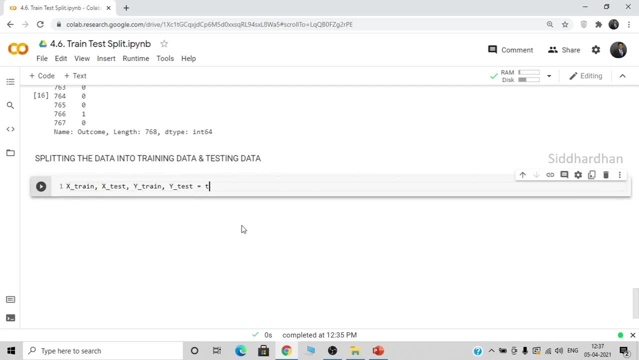 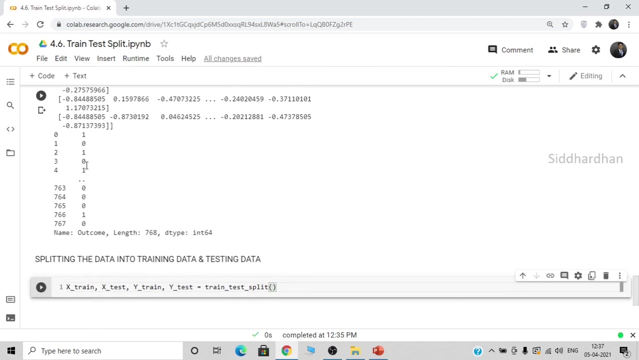 is meant by these four arrays. so in a moment, so before that, let me complete this line of code. so train test split, and inside this train test split function we need to mention the parameters. so here we need to need to to mention x and y. we know that x are the features and y are the outcome, so we need to split this x. 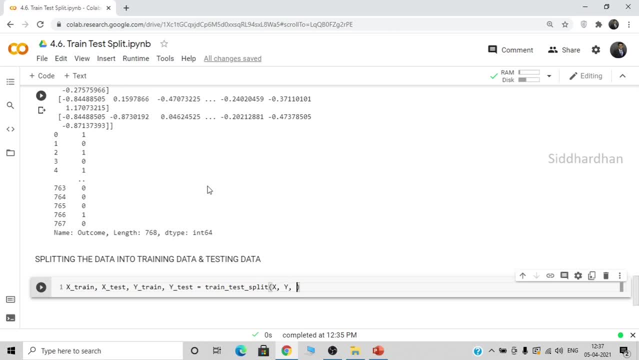 and y, so we need to mention x and y, and then let us mention the test size. so test size is equal to 0.2. okay, so 0.2 means i want to take 20 percentage of the entire data as test data. so, as i have told, 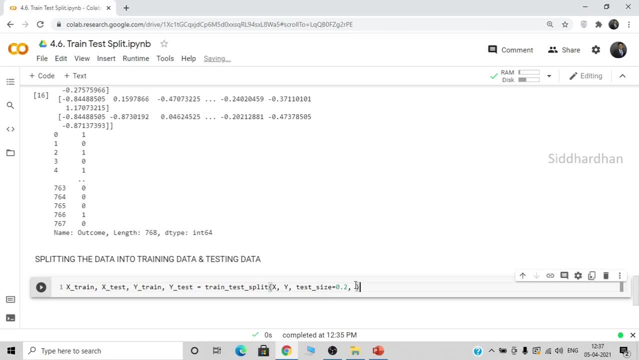 you earlier during the presentation that we take either 10 percentage or 20 percentage of data as the test data, right? so in this case i'll take 20 percentage of data as the test data and then i'll mention another parameter, which is random state. okay, so let me put: random state is equal to 2. 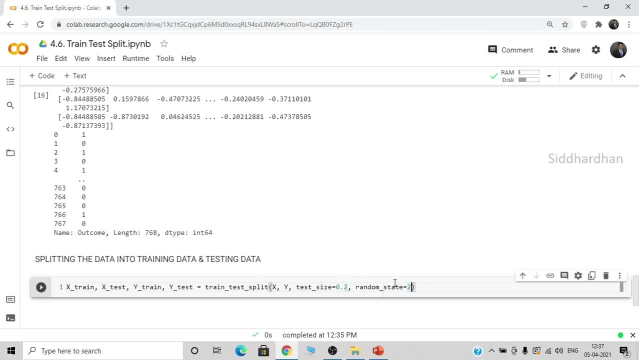 so you can give any integer values for this random state. so the reason for this is: if you want to split the data the same way that my data is getting splitted, then we need to give the same value here. okay, so if you give the value as 2, your data will be splitted in the same way that my data is going. 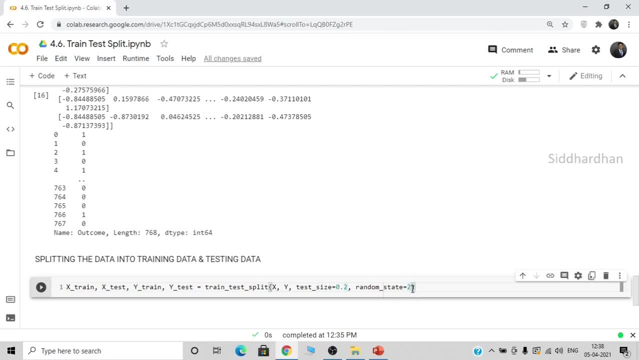 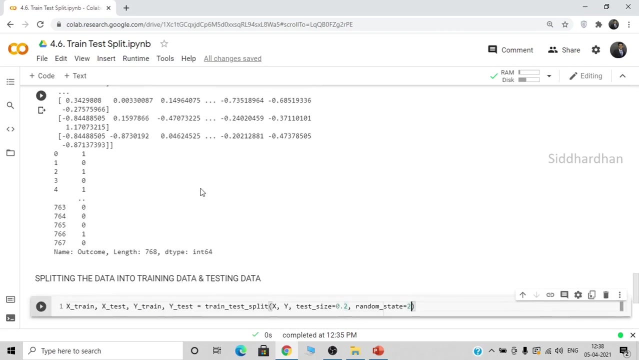 to get splitted. okay, so if you mention 3, then your data will be splitted in a different manner. okay, so these are the parameters which we need to mention: x, y, test size and random random state. okay, and now we have this: four arrays. so extreme is nothing, but this features. okay, so these features will be splitted. 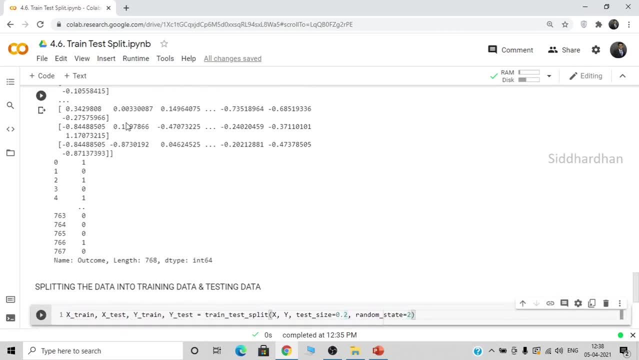 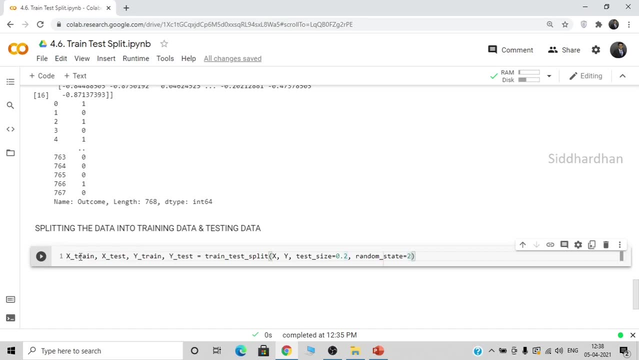 into x train features and x test features. so 80 percentage of the data points in this features will go into this x train and 20 percentage will go into this x test and the corresponding labels of this x train will be given to you. okay will be, you know, going into this y train array. okay, so this corresponding y will be splitted into.